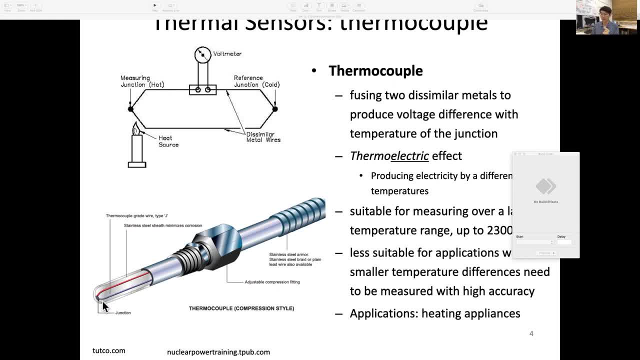 you can see this red and blue metal wire and they have a junction And that junction is a sensing point and it will generate for voltage. So this one is suitable for measuring over large temperature difference, such as up to several thousand degrees, And 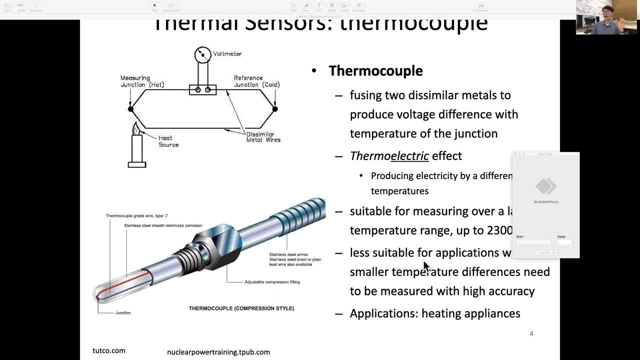 so, on the other hand, it's less suitable for where very small temperature differences need to be measured with high accuracy. So that is less likely and this application is more like heating appliance. So you know, if you have a heating appliances such as rice cooker at home, and it's likely- 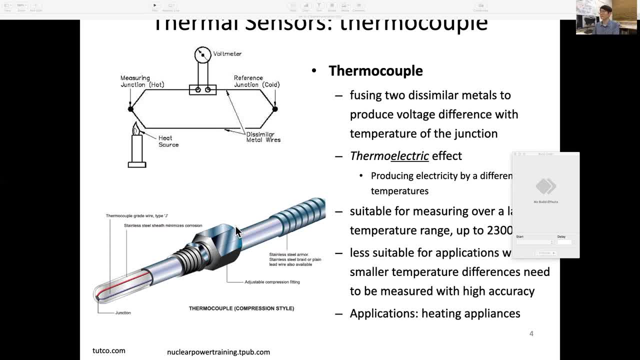 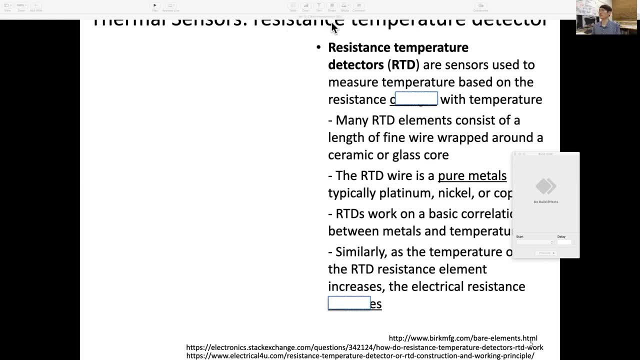 that this thermocouple has been used. And the second is: I want to introduce this so called RTD element, which is Resistance Temperature Detector. So these RTD are sensors used to measure temperature based on resistance changes with temperature. And how does this RTD, or Resistance Temperature Detector, looks? It's a very fine wires wrapping. 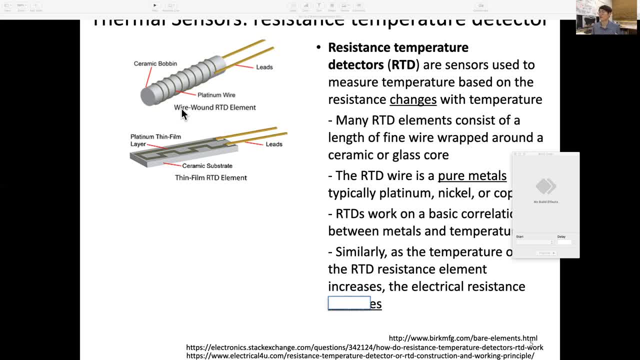 around a ceramic or glass core. So here's the two examples, with this ceramic very fine wires wrapping around. So when the temperature changes and these substrate thermal expansion will affect the wire, Then it can be used for the temperature changes sensor. So this one is a platinum thin film. 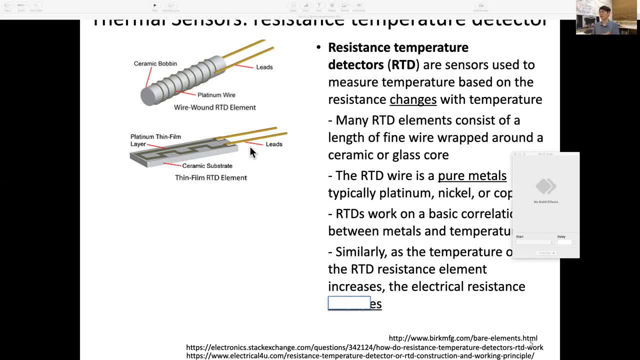 layer with on the ceramic substrate and there's a lid. So this RTD or Resistance, Temperature Detector wire is usually a pure metals, typically platinum, nickel or copper. So so this resistive, resistive, resistive, resistive. 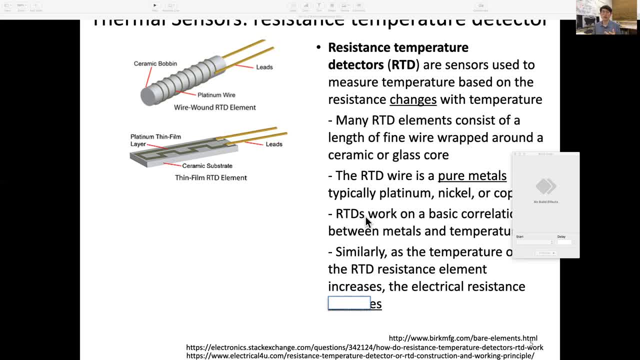 resistive, resistance, temperature detectors working on a basic correlation between these metals and the temperature, And so it looks almost like this ceramic and this is a thin film, And so let's see the this actual data. So when the temperature rises, thinking about this, the relative resistance. 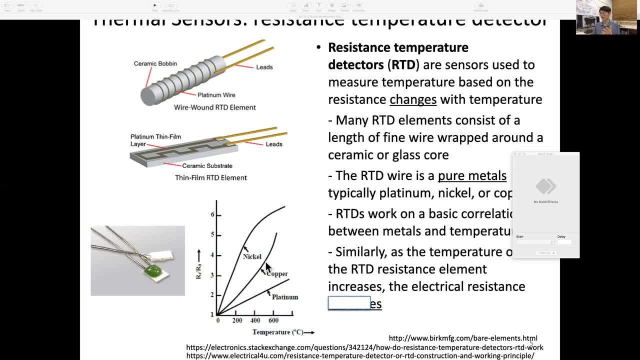 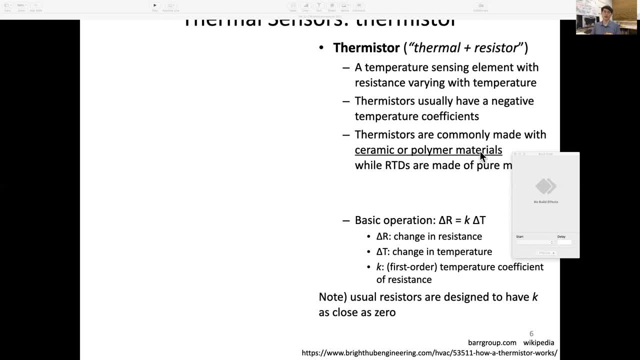 So this is my theory on this. so that ceramic or glass substrate were thermal expand when the temperature rises, and this is a very thin wire, will also elongate, so theคะ POPE would also increase. Alright, Okay, so now? Alright, so you vast- This is my theory on this- so that ceramic or glass substrate were thermal expand when the temperature rises, and this is a very thin wire, will also elongate, so the diameter or cross section will increase. 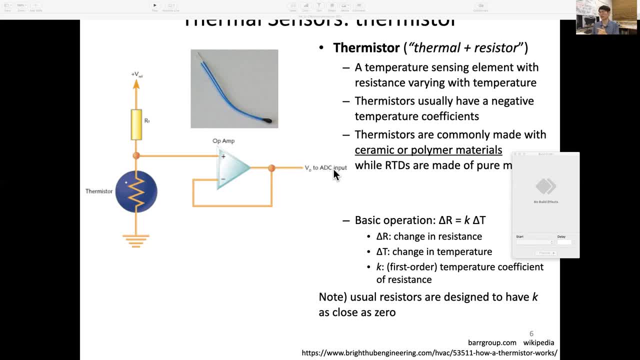 analog to digital converter as an input. So this needs a circuitry. that you see this thermistor, When the temperature changes, this resistance changes And you see this is a voltage reference and this RT and this thermistor resistance is a voltage divider, and that you measure it. 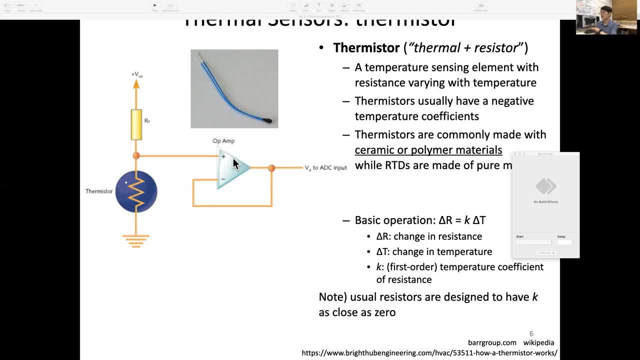 with this voltage follower. So the basic operation is resistance changing is supposed to be related to temperature change, with a constant as a first order. So look at these data. compared with RTD versus thermistor, You see much large resistance changes. you can see. 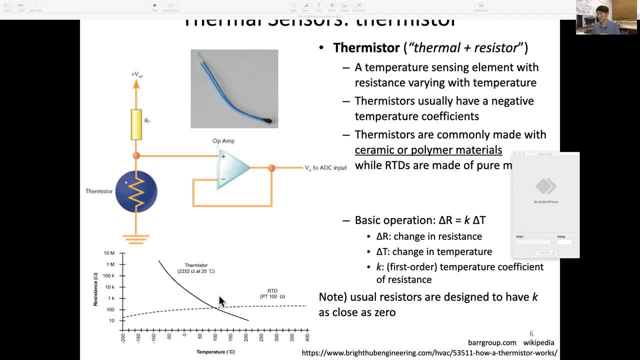 So it has a higher gain or sensitivity and also gives you a higher sensitivity. The slope is opposite. So then, when temperature rises, these thermistors resistance actually goes down And for, as a note, that typical resist registers which you don't want, it change its resistance over time. 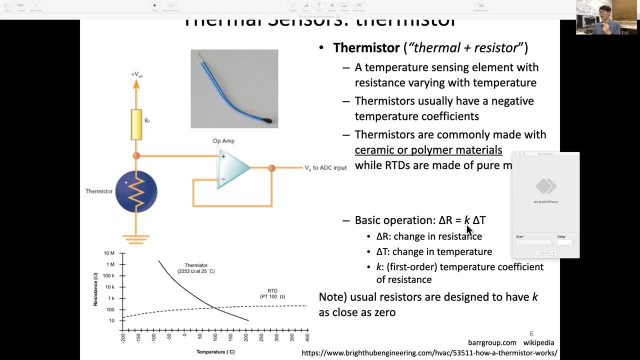 So these are designed to have K as close to as zero. but in thermal sensor or thermistor you want the K as big so that it can be more sensitive. So to describe this, people have developed this empirical formula too, And you can, at a certain temperature. 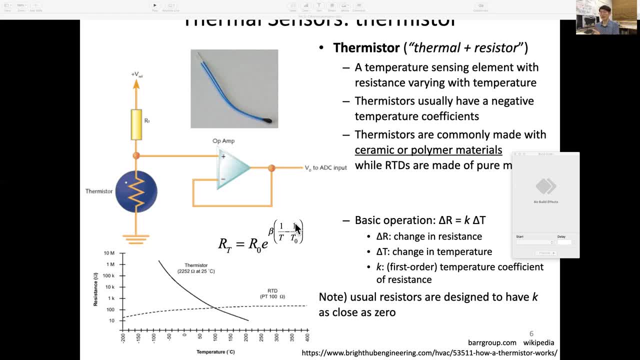 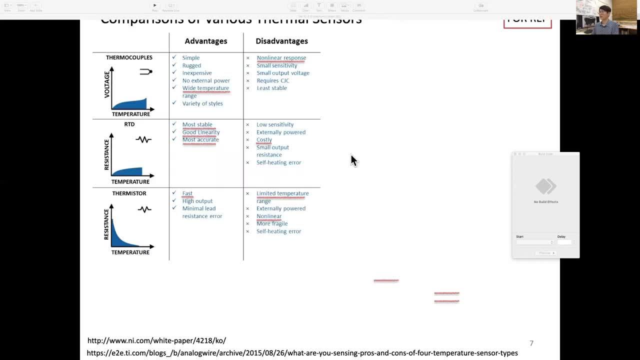 you can always normalize this by Taylor series expansion and you can make a linear approximation. So let's compare these various thermal sensors- And I note here what's worthwhile to note- and thermocouple and resistance, temperature detector, resistance thermal detector and thermistor. 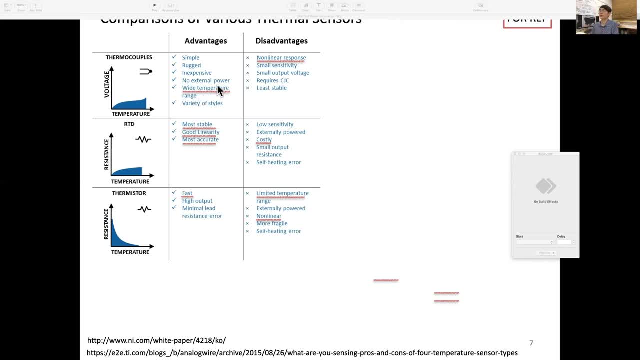 And thermocouple is a can measure wide range of temperature. but why it's nonlinear? Let's see the data. So thermocouple, you see it's a little bit nonlinear and RTD is more stable, very good linearity and the most accurate wire. 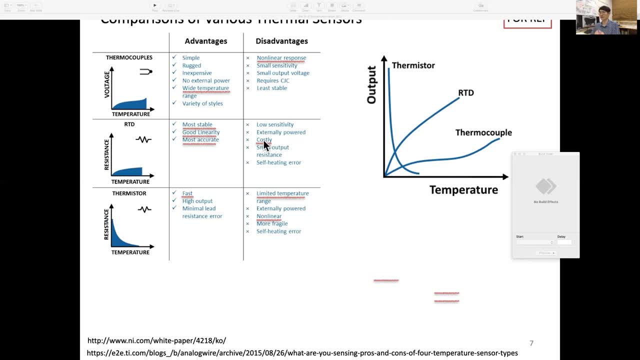 You know it requires a pure metal, So it's costly. and the manufacturing is difficult, So it's costly. And while thermistor is a very quick, fast based on the sensing element as a polymer, while you can see the range of temperature limited, 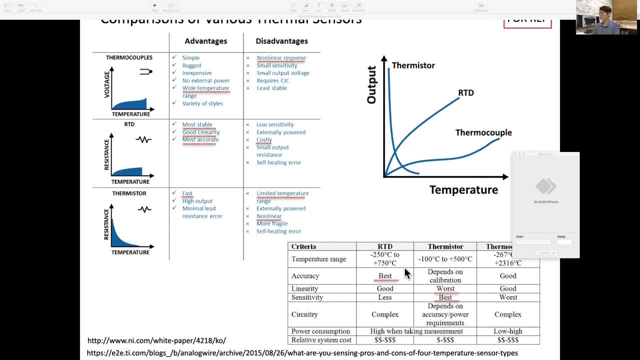 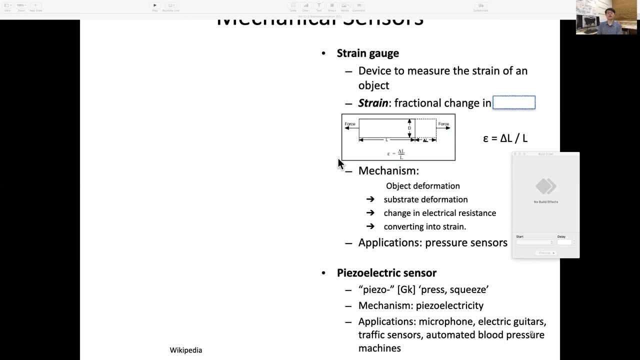 and itself is nonlinear response. So there's another comparison chart for range and accuracy, linearity and sensitivity. You can take a look. So now let's move on to discuss about mechanical sensors- Usually mechanical sensors. we're talking about strain gauge. 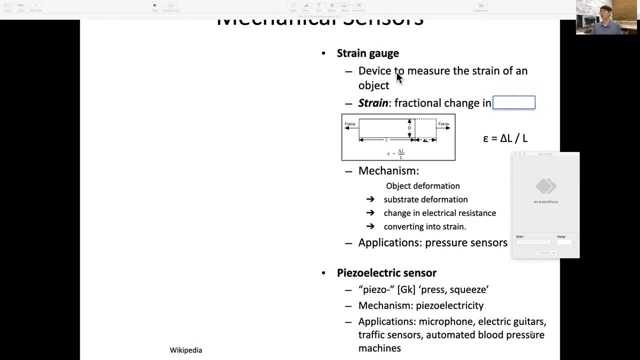 and what are strain gauge and what is strain. So we need to define and the strain first. So when there's a mechanical element and let's say you pull this element with a force, then it's likely to elongate. So it'll elongate based on original length of air. 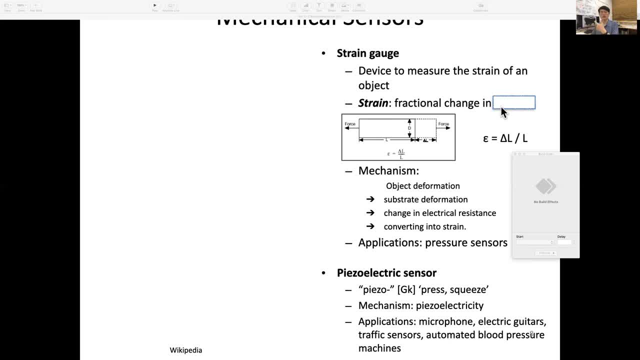 at the change as a Delta air and the fractional changes in length. So it's a unit list and that's defined as a strain. You can see a strain as an epsilon equals Delta air over air sub zero. okay, So the device to measure strain of an object is called strain gauge. 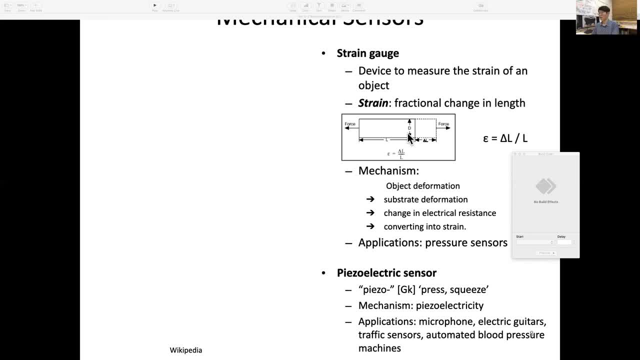 And how we can use this. So let me first show how strain gauge it looks like. So this is on a thin film. These are resistance element like that And usually, in this case, measures. this ups and downs the strains And deformation of this object. 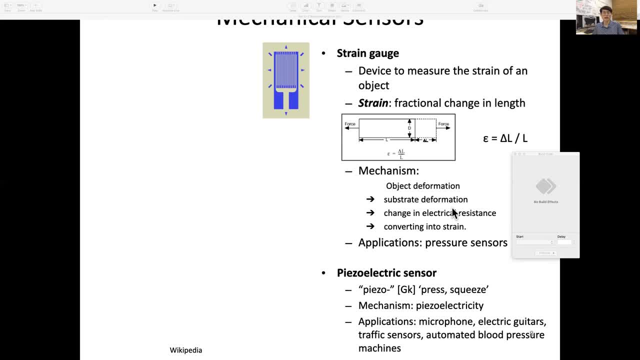 gives a substrate deformation and that results in changes in electrical resistance And you can convert that resistance change into the strain gauge, strain. so let me give you a an example: pressure sensors. so you like music and guitar, like electric guitar, these piezo, electric, not piezo, it's a strain gauge. 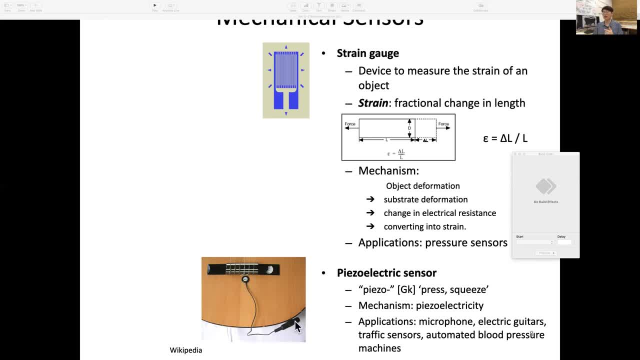 it's used here to detect and amplify and converting this sound into an electric signal, and the mechanisms are pretty simple. you see, these are actual ones- into a cartoon. then strain sensitive pattern. you, in this case you see this directional change. so that's more like this directional strain we are measuring.